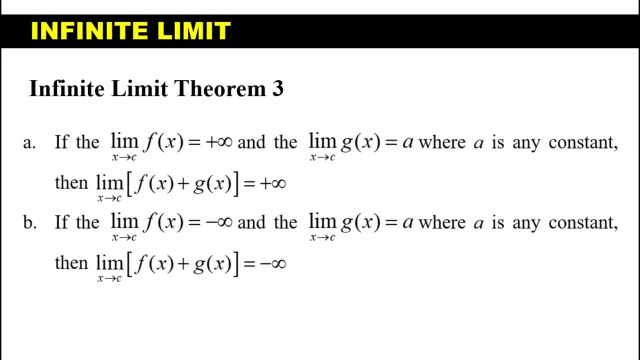 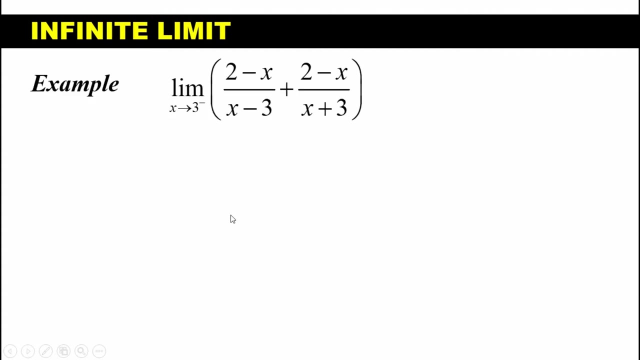 of x as x approaches, c is negative infinity. Now, since we do not know how large positive infinity or how small negative infinity is, whatever constant you add or subtract to positive infinity or negative infinity, the answer will always be positive infinity or negative infinity. So say, for example, we have the limit of 2 minus x over x minus 3 plus 2 minus x over x plus 3, as 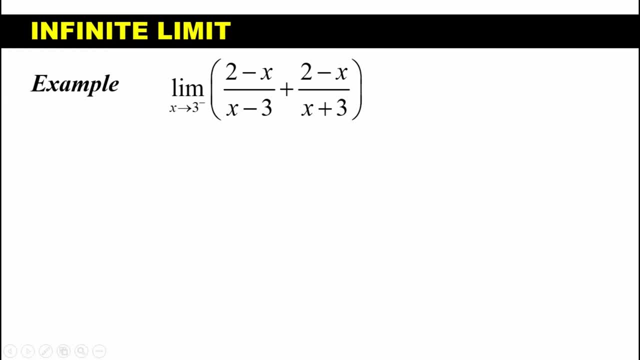 x approaches 3 from the left. Now if we try to solve for their individual limits, we get the limit of 2 minus x over x minus 3, as x approaches 3 from the left is positive infinity. Why do we get positive infinity If we substitute? 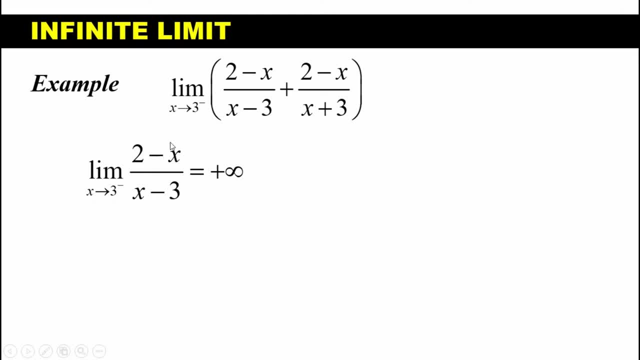 3, this will become 2 minus 3. this will become negative. 1 negative. 1 divided by negative is positive. we have positive infinity. Now for the next function. we have the limit of 2 minus x plus 2 minus x, over x plus three as x approaches 3 negative. Now if we substitute 3 to the function, 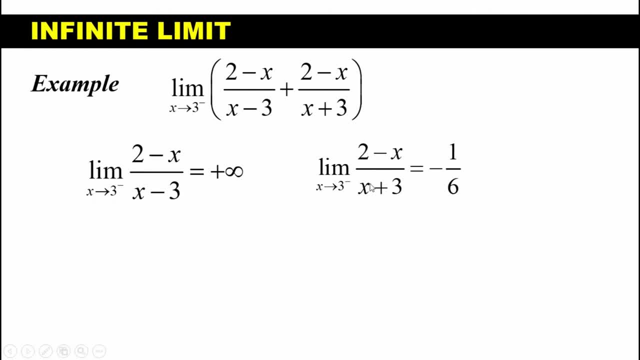 we have: 2 minus three is negative 1, and then 3 plus 3 is positive, 6 negative 1 divided by positive 6 is negative 1 over 6. now if we try to solve for the limit of 2 minus x over x minus 3 plus 2 minus x, 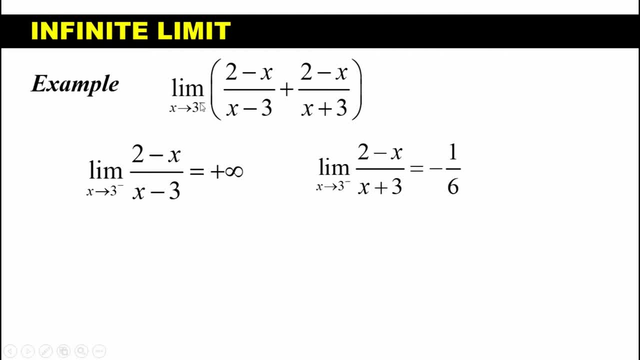 over x plus 3 as x approaches 3.. 3 from the left, since we already have their individual limit, so we can have the limit of positive infinity minus 1. sixth, as x approaches 3, negative and if we simplify that one, since this is positive infinity, whatever value of our constant is, as long as this is positive infinity. 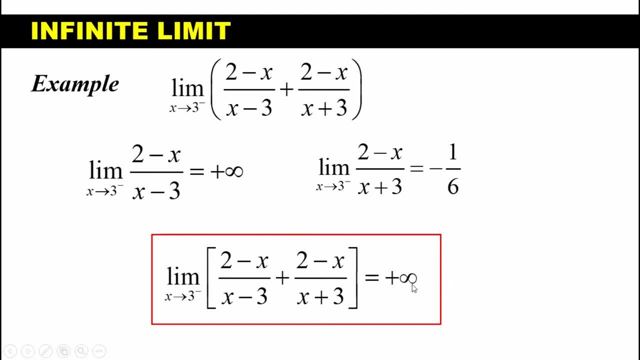 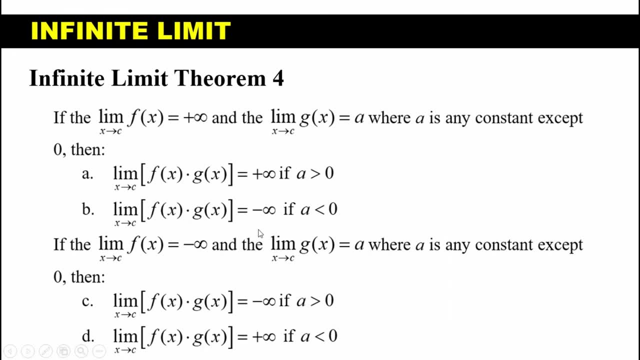 the answer will always be positive infinity. now let's move on to infinite limit, theorem number 4. according to infinite limit, theorem number 4, if the limit of f of x is positive infinity and the limit of g of x is equal to a, where a is any constant except zero, then the limit of f of x 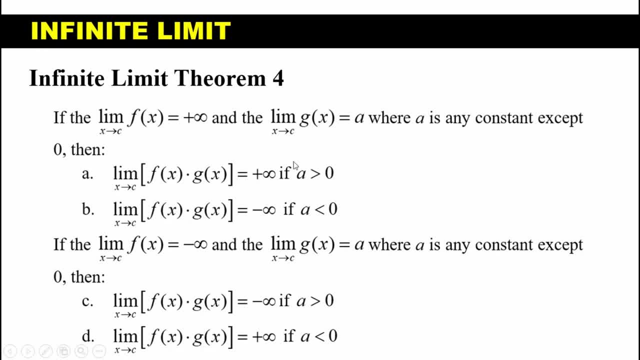 times g of x as x approaches c is positive infinity if a is greater than zero, and the limit of f of x times g of x as x approaches c, if is equal to negative infinity of a, is less than zero. another is: if the limit of f of x as x approaches c is equal to negative infinity, and. 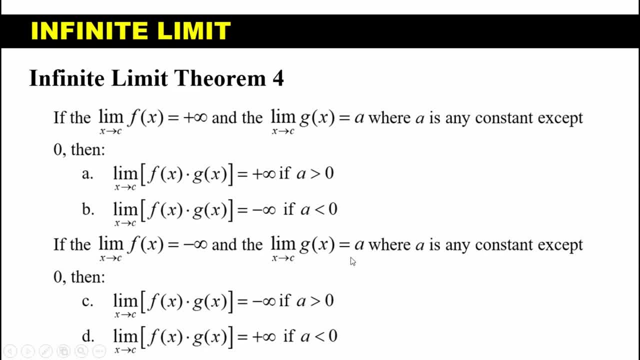 the limit of g of x as x approaches c is equal to a where a is any constant except zero. then the limit of f of x times g of x as x approaches c is equal to negative infinity if a is greater than zero and positive infinity if a is less than zero. so there are four conditions that we need to understand and consider. 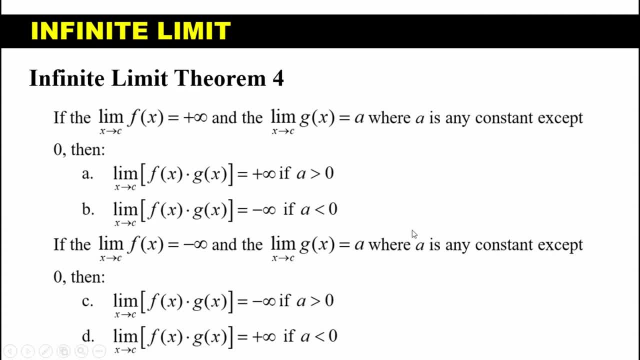 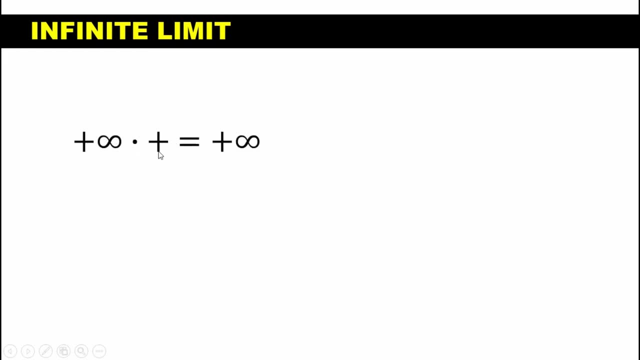 and just like infinite limit, theorem number two. this might be a little hard to understand or memorize, but to understand it simply, let's put it this way: say we have positive infinity and you multiply that one with positive value, the answer is, of course, positive infinity. positive infinity times negative. the answer is negative infinity if you have negative infinity, if 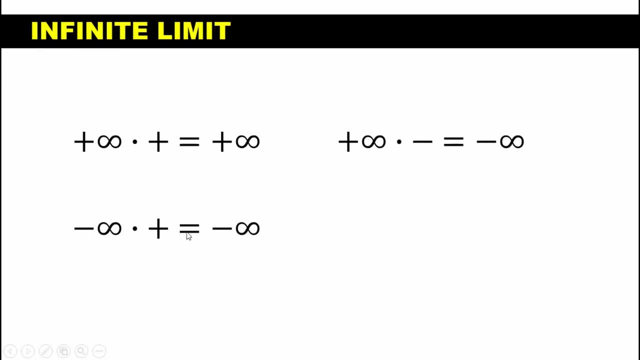 and you multiply that one to a positive value, then the answer is negative infinity, since negative times, positive is negative. now, if you have negative infinity and you have a negative constant value and you multiply them, the answer is positive infinity, since negative times negative is positive. so this is the 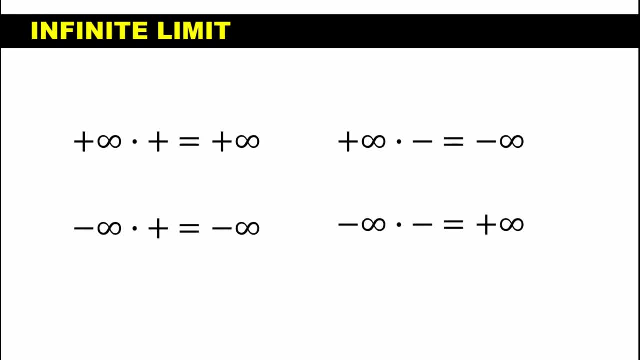 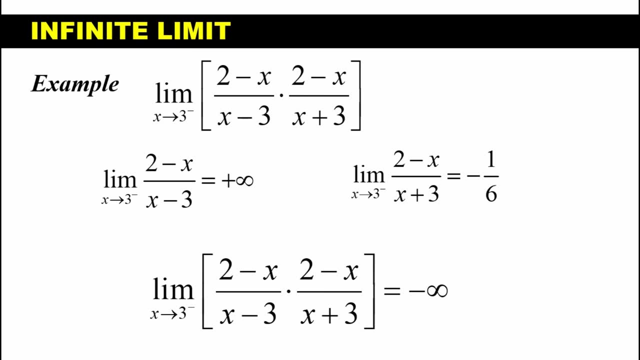 simplified way of understanding infinite limit. theorem number four. now say, for example, we have the limit of two minus x over x minus three times two minus x over x plus three, as x approaches three from the left. now if we look for the limits, the individual limits, we get positive infinity. and 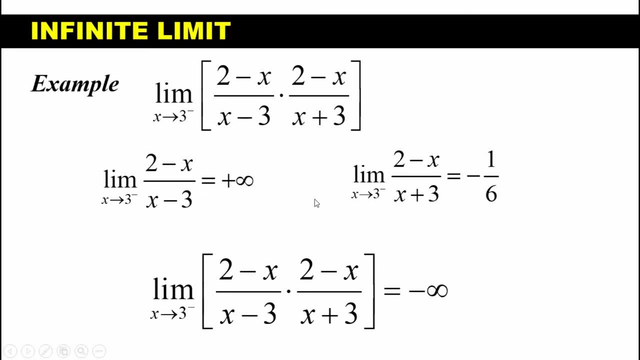 negative one. sixth, the same with our previous example. now, since we have positive infinity and we multiply positive to a negative constant, since this is positive, this is negative positive times, negative is negative infinity. another example is the limit of 3x over x minus 5 times 3x over x plus 5, as x approaches 5 from the left. now pause this video.